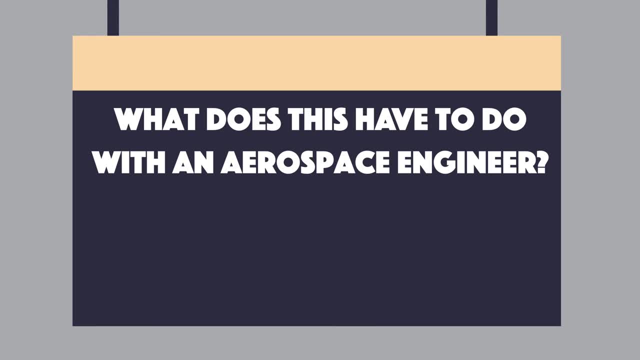 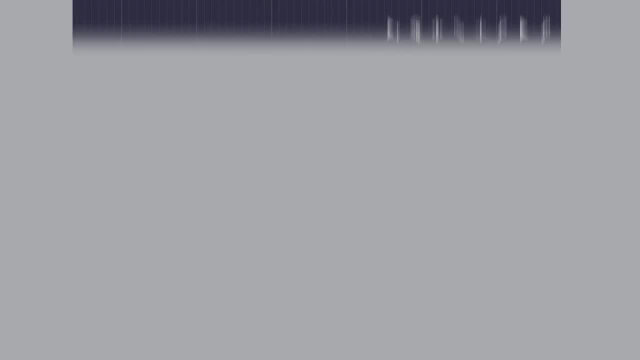 But what does this have to do with an aerospace engineer? They just design and build right? Yes, they do. But they have to know who and what the craft is for. You see, following the horrific accident with the Concorde in July 2000,. 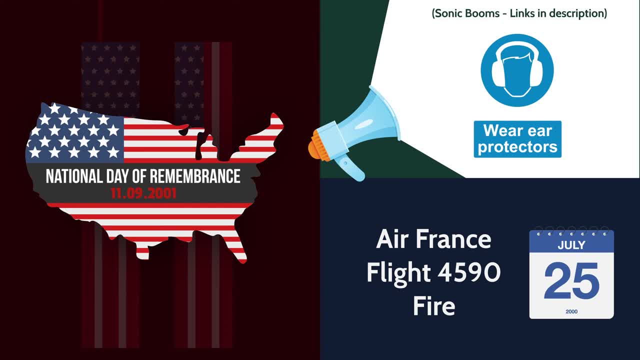 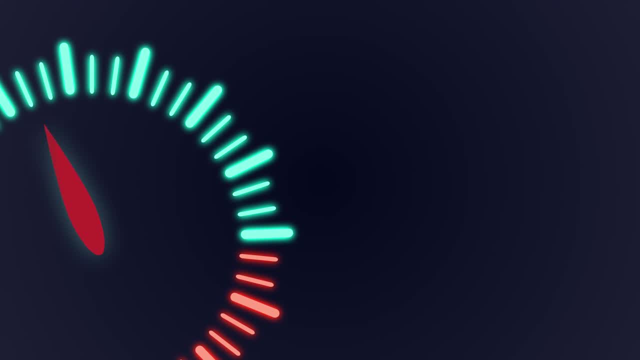 the events from the 9-11 and the deafening sonic booms. what passengers really wanted the most was safety, economy and looking after the environment. So, yeah, getting there fast is important, But so is making sure what you build is needed, And really this is what aerospace engineers need. 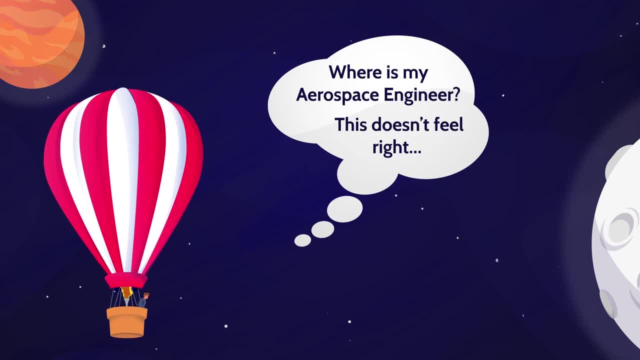 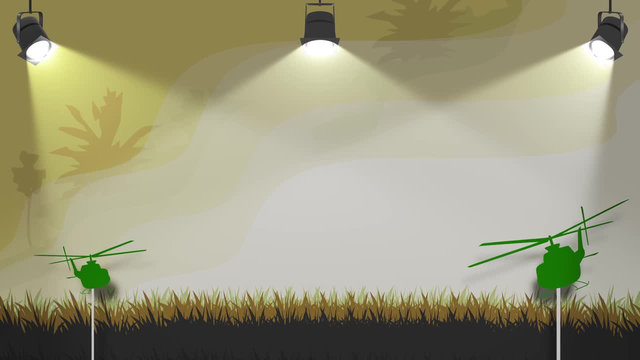 They consistently evaluate and assess the requirements, looking holistically at the design, who it's for and specifically. why. Take military aerospace engineering, for example. Here the requirements are completely different. The importance for the environment and cost isn't high on the list. But the quality and safety of the pilot and the plane is crucial. The craft is engineered completely differently. I mean it can get from NYC to LA in 40 minutes, but who wants to arrive in LA after exerting nearly 9 Gs with no luggage? 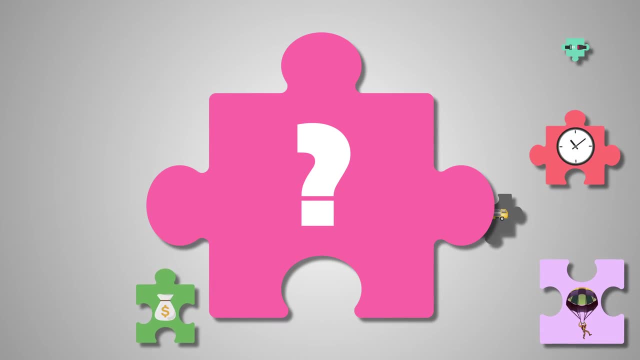 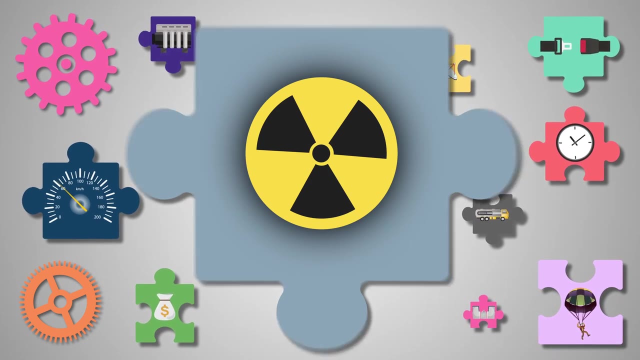 It's not really suited for that. So how exactly do they think about all of this? Well, for them, it's about solving one problem at a time. For example, one of the biggest issues with space travel is galactic cosmic rays. 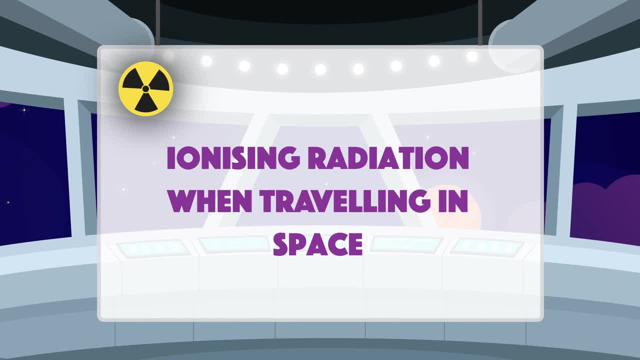 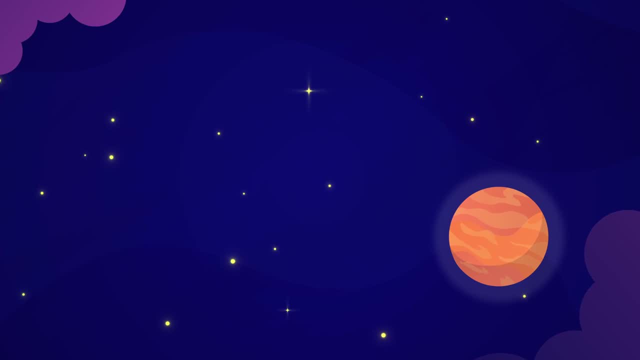 Basically ionising radiation when travelling in space. Now, on Earth we are protected by our atmosphere, But in space there's very little but the spacecraft protecting you from this radiation. So it's thinking about new material that could be used that isn't heavy and inefficient like lead. 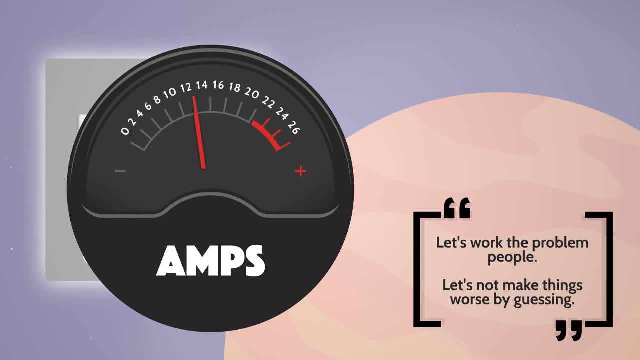 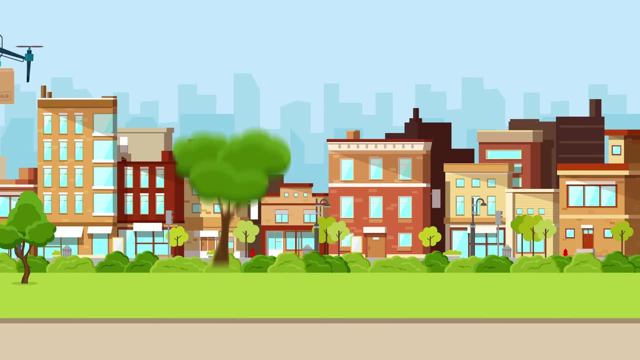 The next problem: Power and fuel. We've all seen Apollo 13.. Back down to Earth, Amazon wants to take their prime services up a notch and drop off your parcels with drones. Sure, they have years left of testing, but what problems are they solving? 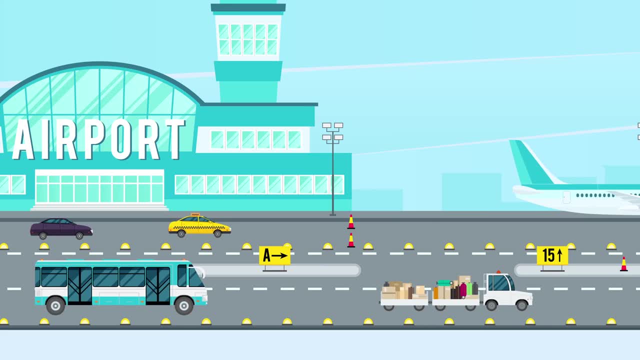 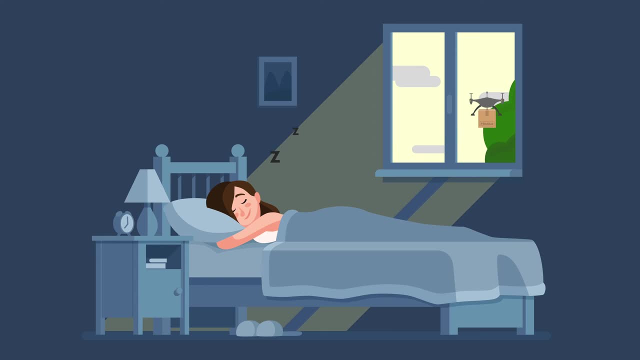 Think about the integration with commercial airspace. or even the public. What would the public think about drones flying everywhere? Would you be happy with one hovering outside your bedroom at 7am in the morning? Depends, if it's your parcel, I guess. 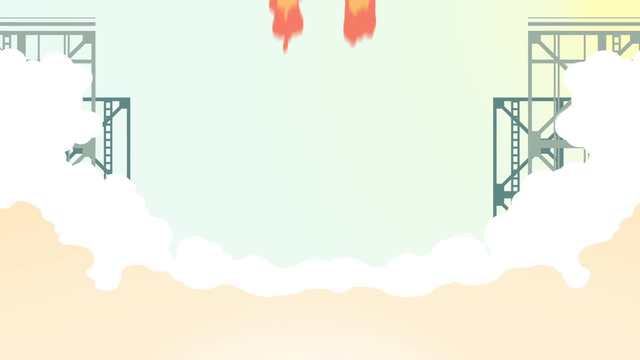 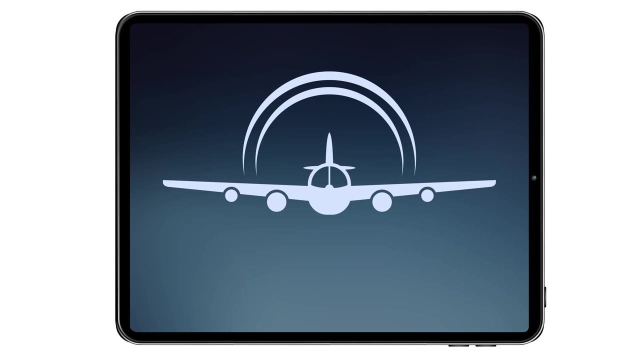 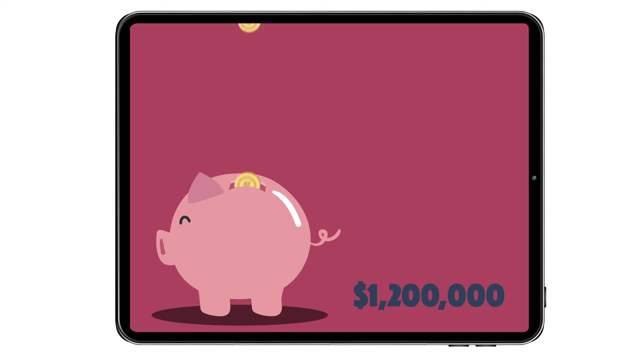 But it doesn't always have to be about implementing extraordinary features of engineering. One firm decided to replace their pilot's paper manuals, which consisted of logs, maps, safety manuals, and replaced it with an iPad, Savings $1.2 million in gas costs alone, not to mention the safety improvements.